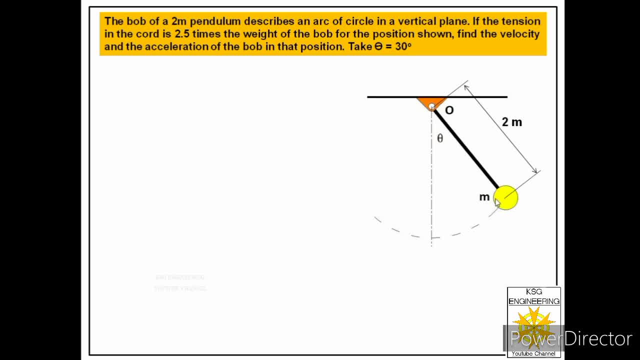 find the velocity and acceleration of the bob in this position. And it is mentioned that tension in the chord is 2.5 times the weight of the bob for the position shown. So let us solve this problem now. So the very first step is we have to draw free body of. 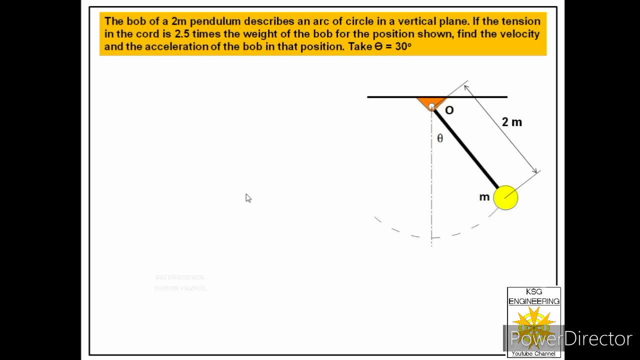 the bob In order to draw free body of the bob. first of all, we will represent that bob on paper And we will show two directions for that bob. One will be tangent to the path. Second is normal, to the path that is directed towards the center. So we have shown those. 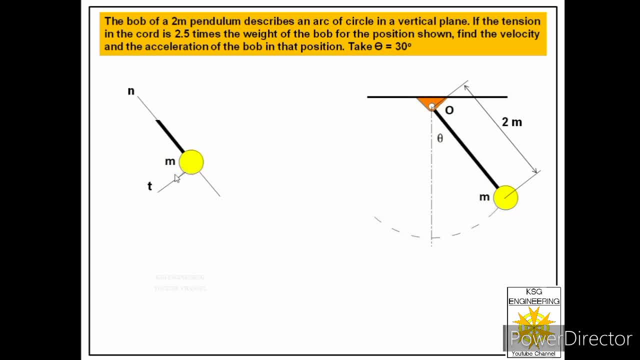 two directions. One is tangent to the path. Second is normal to the path that is directed towards center. So this is tangential direction, This is normal direction. Now let us see what forces we have to represent in the free body of this bob. So the first force will be the. 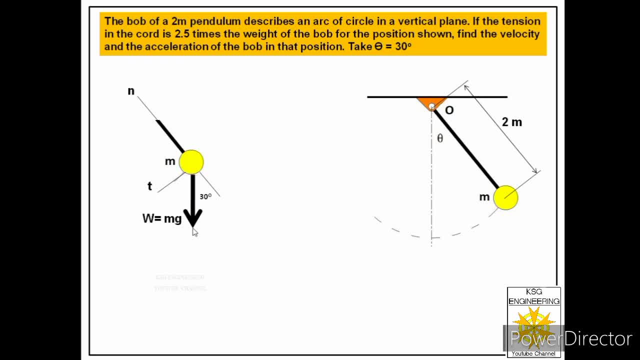 weight of the bob, Which will act in downward direction, And we will call it as w equal to mg, Where m is the mass of the bob given to us in this problem And g is the acceleration due to gravity. And this normal is given to us at 30 degrees with the vertical. It means this: 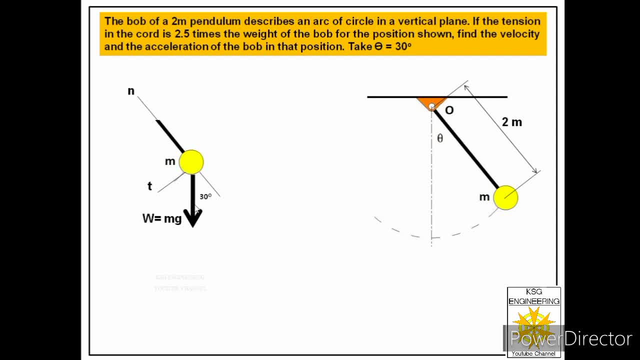 angle will also be 30 degrees, Which this weight will make with the normal. Now the second force which we have to represent in the free body of bob will be the tension in this cable. So in this cable, tension will act towards the center And we will label. 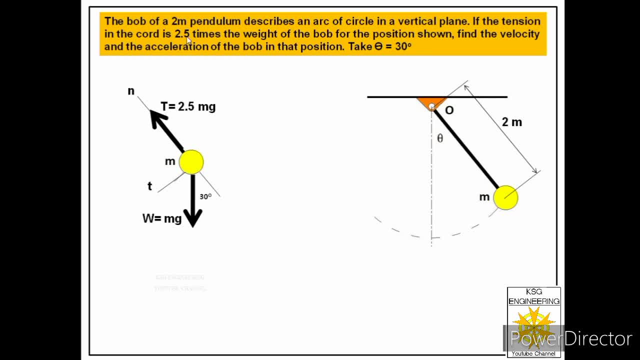 that tension as t, And it is mentioned in the problem that tension in the cable is 2.5 times the weight of the bob And we know weight of the bob is mg. So we have represented t is equal to 2.5 mg. Now these are the forces acting on the bob And we know bob is in motion. 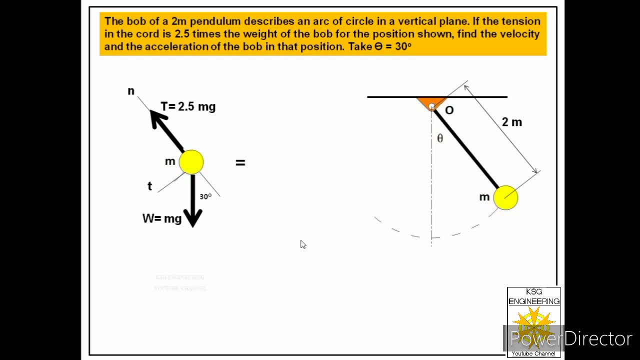 So these forces are responsible for two types of acceleration of the bob. One will be the tangential acceleration, Tangent to the path, And second will be normal acceleration that is directed towards the center. So we will say: Summation ft. 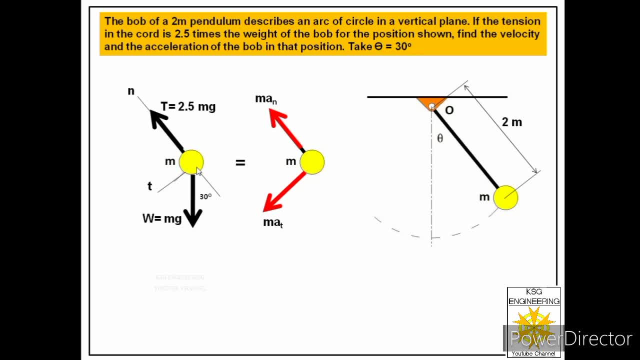 Means sum of the forces acting tangentially to the path will be equal to mat. Then we will say summation fn, That is, sum of the forces acting along the normal, will be equal to man. Now let us use these equations one by one. So let us first use summation: ft is equal. 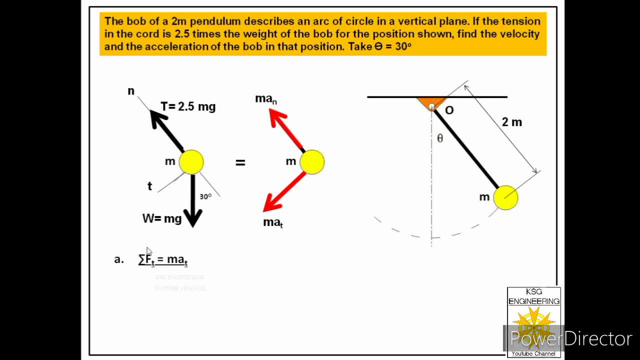 to mat. Now let us see how many forces are in the normal. So the first two forces are acting along tangent to the circular path Over here in this free body. we have two forces. One is acting along normal And second is acting at some angle to tangent and to normal, And it has angle of 30 degree with the normal. 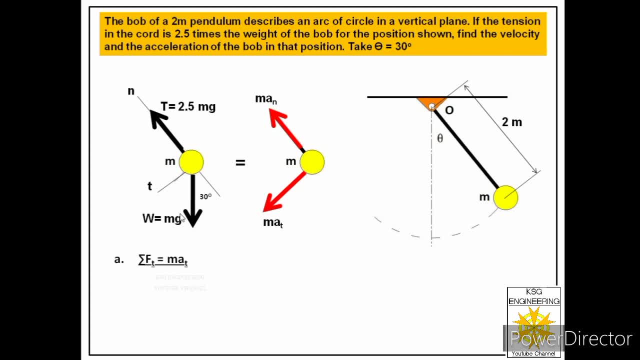 It means we have to resolve this weight into its components. So This cos component, this will be sine component. so along normal its component will be mg cos 30 degrees and along tangent its component will be mg sine 30 degrees. it means in this free body we have only one force acting tangentially. 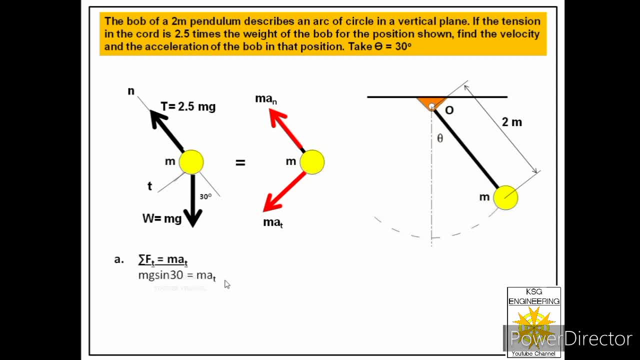 to the circular path. so that is mg sine 30 and it will be equal to M 80, where M is the mass of the Bob, 80 is the tangential acceleration of the Bob. so from here M will cancel out and we will get tangential acceleration of the Bob. 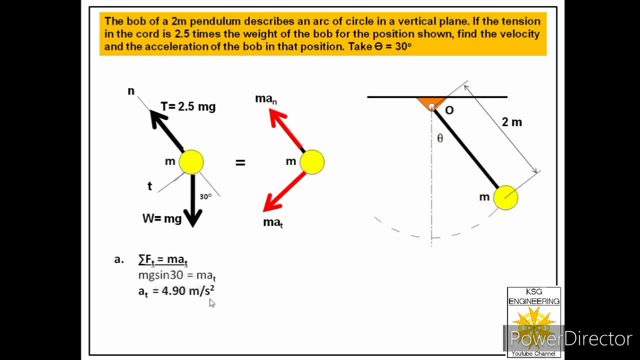 as 4.90 meter per second square. so we have got our first answer. now we will apply the second equation, that is, summation. Fn is equal to Man. now let us see how many forces are acting along the normal. there are two forces. one is the tension T, which is equal to 2.5 mg, and second is